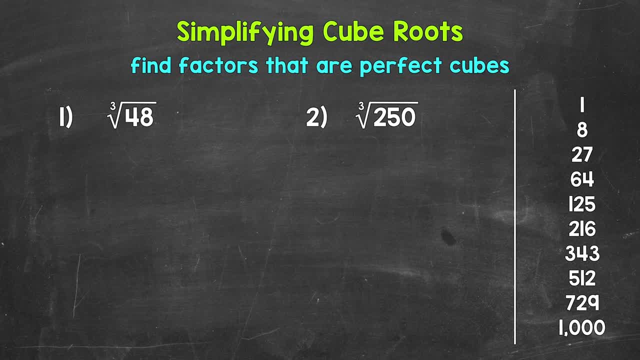 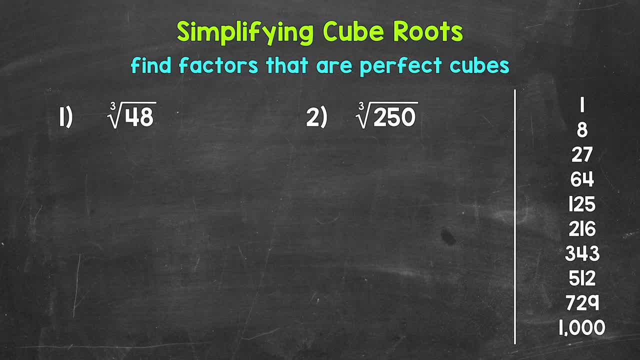 the right I have the first 10 perfect cubes. Knowing and being familiar with these, or as many of these as you can, will make simplifying cube roots and working with cube roots in general much easier. So are any of the first 10 perfect cubes a factor of 48?? Yes, 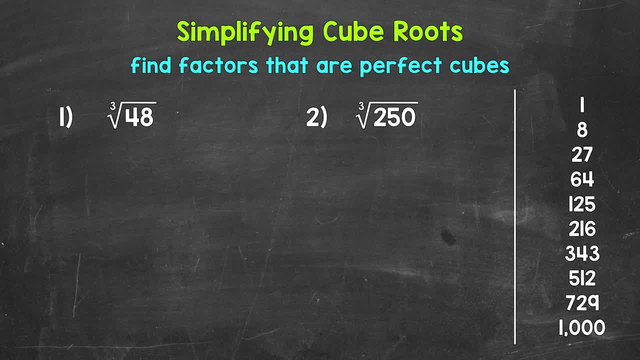 8 is a factor of 48. We know that 8 times 6 equals 48.. 8 and 6 are factors of 48. They go into 48,, so to speak. So let's rewrite the cube root of 48 as the cube root of 8 times 6.. Now the 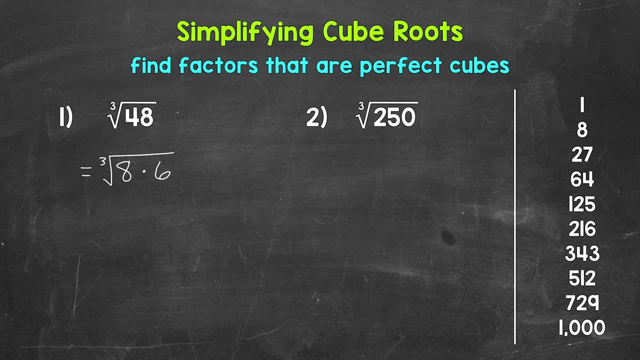 multiplication or product property of cube roots. lets us split this into the cube root of 8 times 6.. Now the multiplication or product property of cube roots. lets us split this into the cube root of 8 times 6.. the cube root of 6, meaning we have the cube root of 8 times the cube root of 6.. This is still. 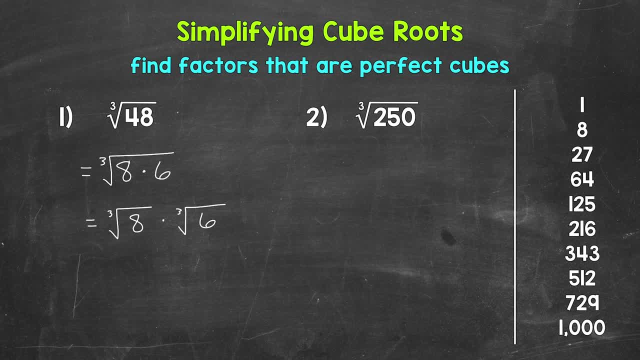 equivalent to the cube root of 48. We're not changing the value of anything at all. Now we can take the cube root of 8, which is 2.. 2 times 2 times 2 equals 8.. So again, 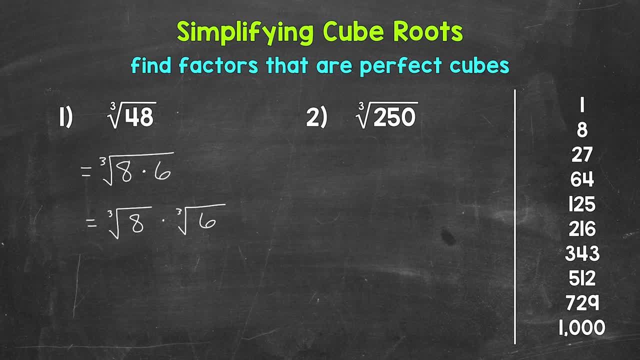 the cube root of 8 is 2.. So we end up with 2 times the cube root of 6.. And that's our final simplified answer. We can't simplify or break this down any further. So again our final simplified answer: 2 times the cube root of 6.. Let's move on to number 2, where we have the cube root of 250.. 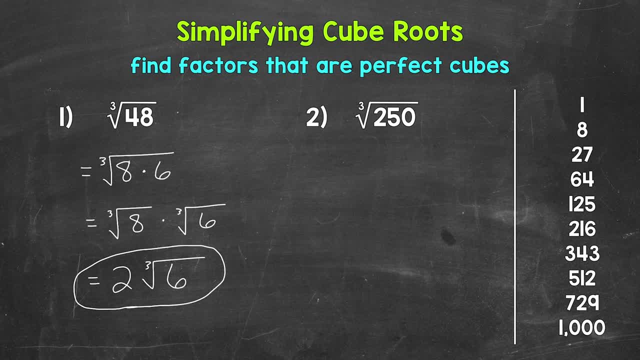 250 is not a perfect cube, but we can simplify. We need to look for factors of 250 that are perfect cubes. Well, 125 times 2 equals 250, and 125 is a perfect cube, Since there's a factor of 250. 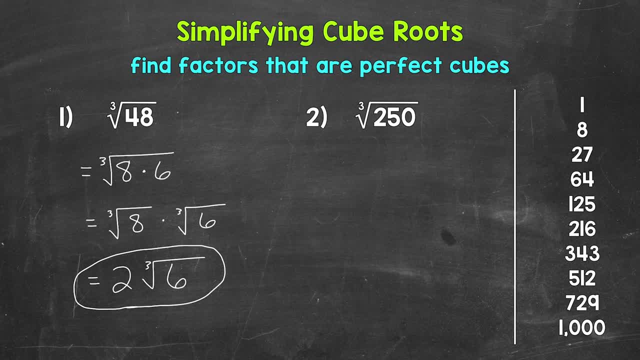 that's a perfect cube. we can simplify. We can rewrite this as the cube root of 100.. 125 times 2.. Now let's split this into the cube root of 125 times the cube root of 2.. Now we can take the cube root of 125, which is 5.. 5 times 5 times 5 equals 125. Again. 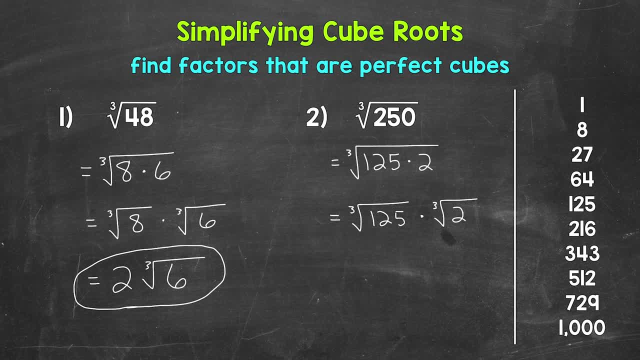 the cube root of 125 is 5.. So this is going to equal 5 times the cube root of 2.. And that's our final simplified answer: 5 times the cube root of 2.. We cannot simplify or break that down any further, So there's how to. 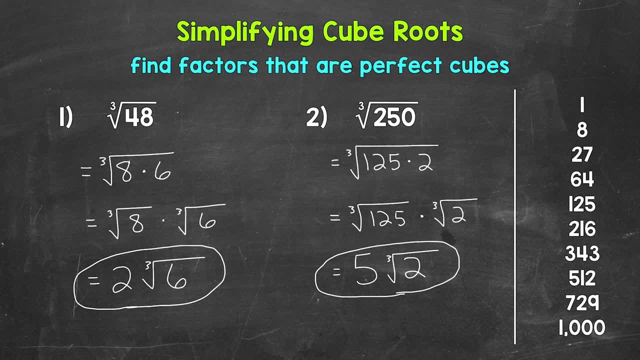 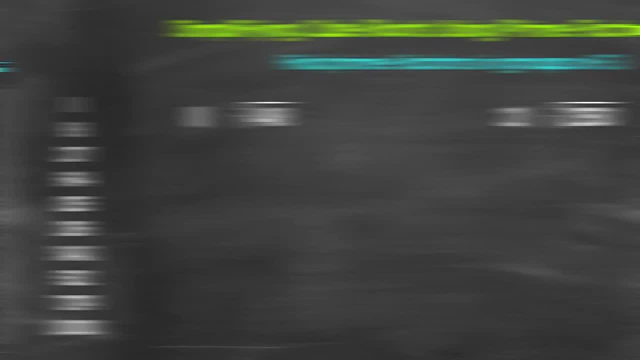 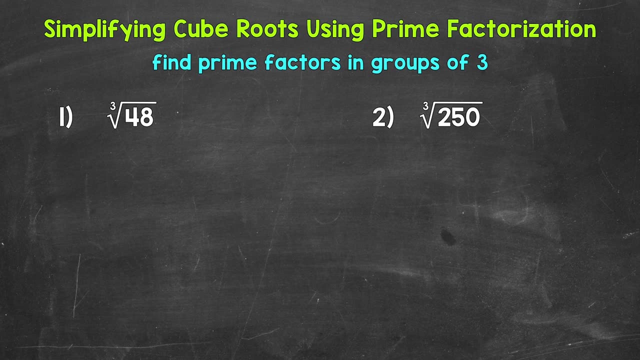 simplify a cube root by looking for factors that are perfect cubes. Let's move on to simplifying cube roots using prime factorization. Here are our examples, and these are the same exact ones we just did. But let's take a look at a different approach. Let's jump into number 1, where we have the cube root of 48.. We're going. 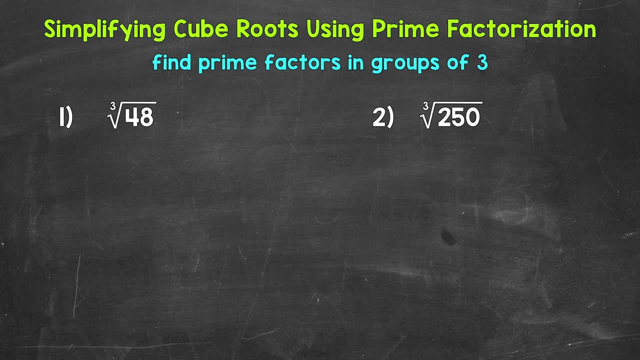 to do this by using the prime factorization of 48 to pull out any cube roots of perfect cubes. So let's start with the prime factorization of 48. We need to break this down. We need to break this down. We need to break this down until we only have prime factors. Now there are different paths to take in order to get to the prime factors, but in the end, no matter what path you take, you'll get to the same prime factors. So something to keep in mind. 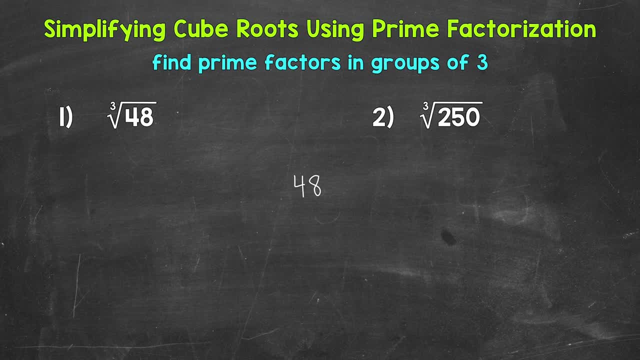 Let's come to the side here and take a look at the prime factorization of 48.. I'm going to start with the factors of 2 and 24.. Now, 2 is prime, so we are done over there and we can continue to break 24 down. Let's use the factors of 2. 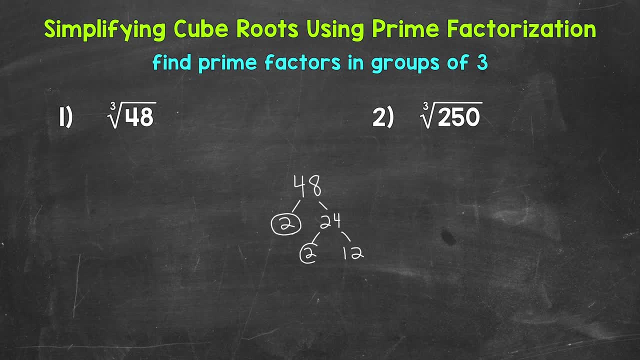 and 12.. 2 is prime, so we are done there. but we can break 12 down. Let's use the factors of 2 and 6.. 2 is prime, so we are done there. but we can break 6 down. Let's use the factors of 2. 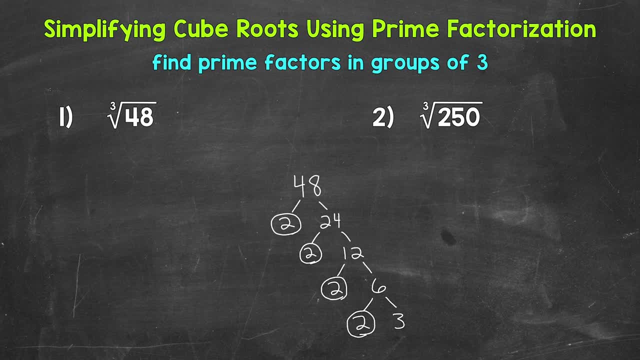 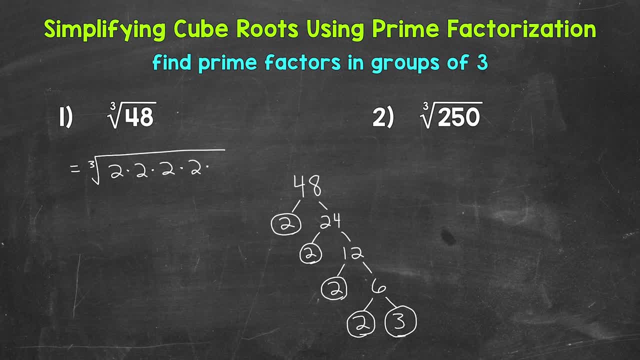 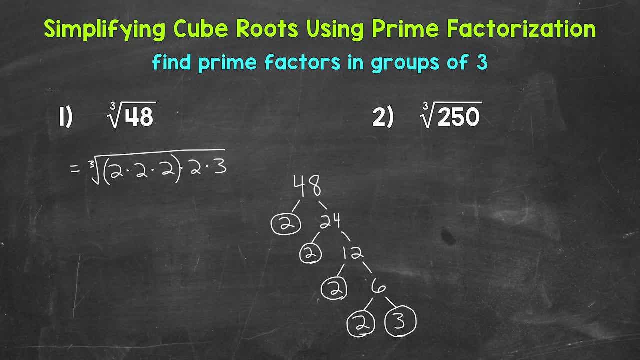 here. That represents a perfect cube that we can pull out 2 times. 2 times 2 equals 8, and the cube root of 8 is 2.. So let's pull out a 2.. So this is going to equal 2 times the cube root of 2 times 3.. We still have. 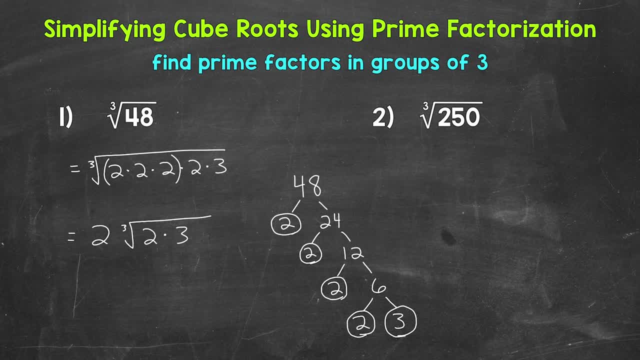 that 2 times 3 under the cube root symbol. We cannot simplify any further, so let's multiply. We have 2 times 3, which equals 6.. So we end up with 2 times the cube root of 6..